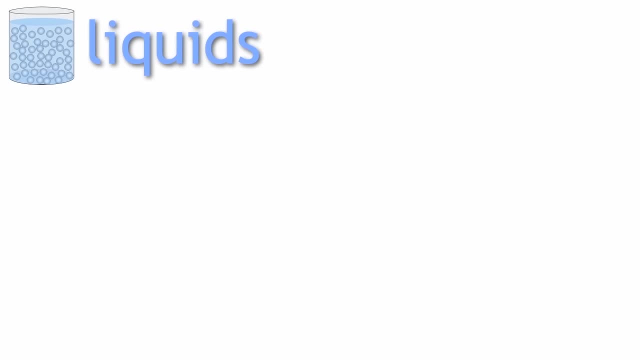 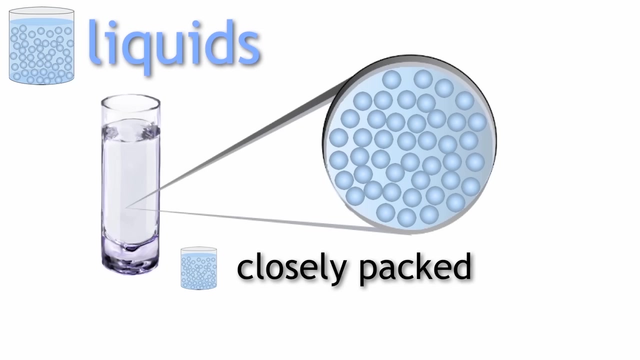 Now let us look at liquids. An example of a liquid is water. Just as with solids, the properties of liquids depend on how the particles in liquids are packed. In a liquid the particles are again closely packed, but not as closely packed as in solids, So this means the particles. 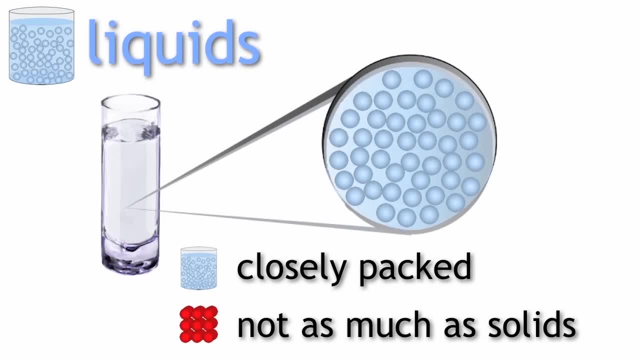 in liquids can move around each other. So liquids are not rigid. but because their particles are closely packed, as in solids, they then move durably into each other. So the particles are not rigid- or was not rigid- so they move around from each other. So these properties 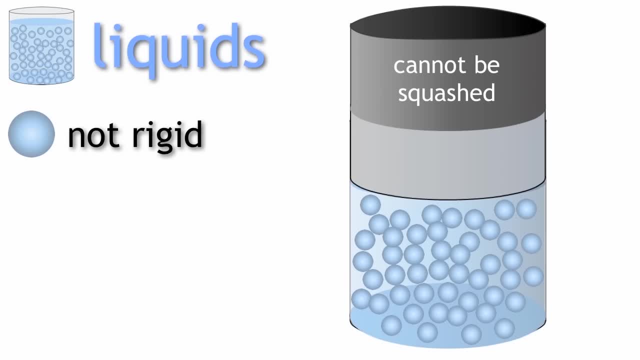 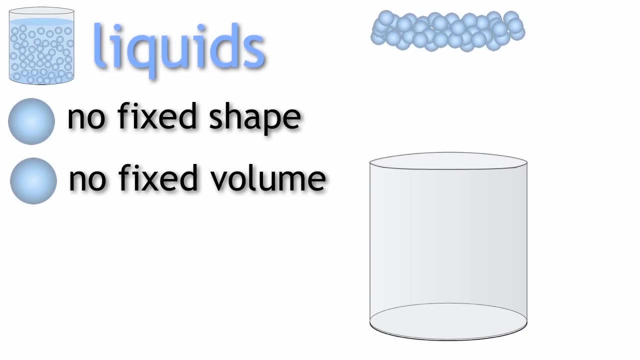 factors in solids. they cannot be squashed or compressed. They do not have a fixed shape, but they do have a fixed volume. Beware with that one, as many students think, because liquids do not have a fixed shape. they do not have a fixed volume either, but they are wrong. 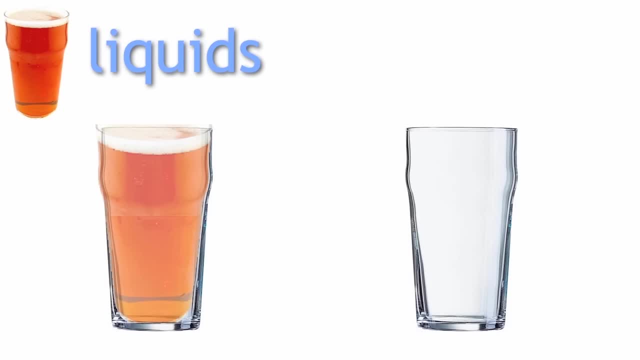 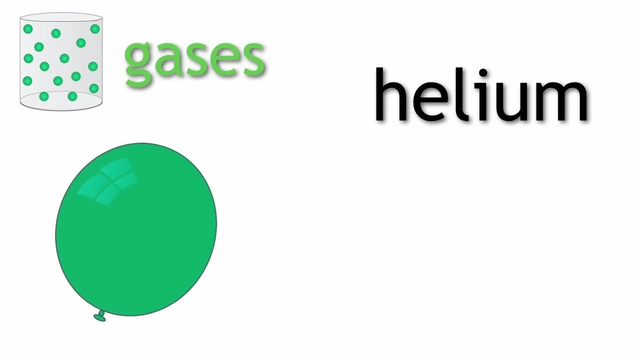 If someone orders a pint of beer, they cannot make it two pints by pouring it into different containers. As you know, liquids can flow. Finally, let us look at gases. An example of a gas is helium. This is the gas in party balloons, because it is less dense than air and unreactive. 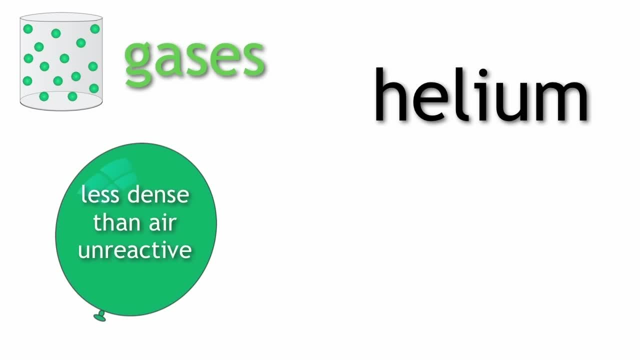 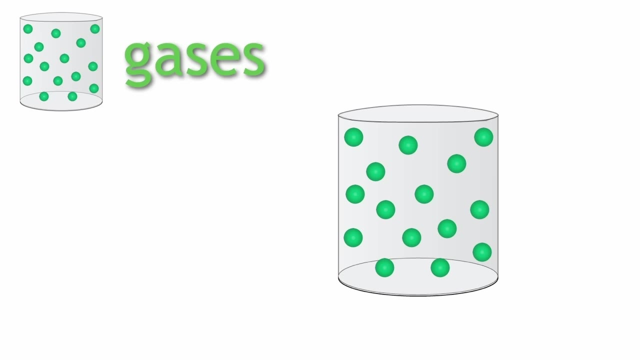 Again, as with solids and liquids, the properties of gases depend on how the particles in gases are packed. Unlike solids and liquids, the particles in gases are not closely packed. Therefore, gases are apart. As a result, gases are not rigid and can be squashed or compressed. 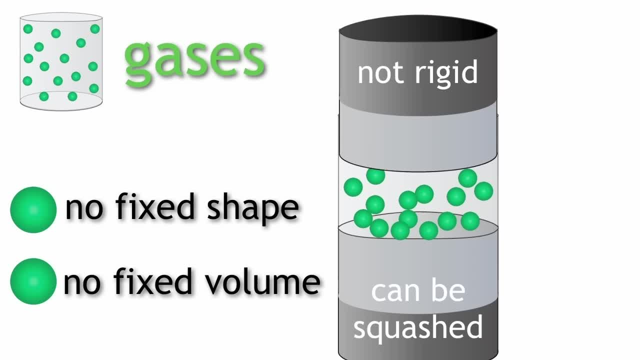 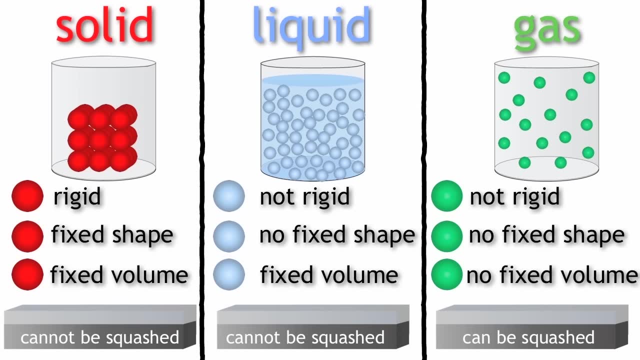 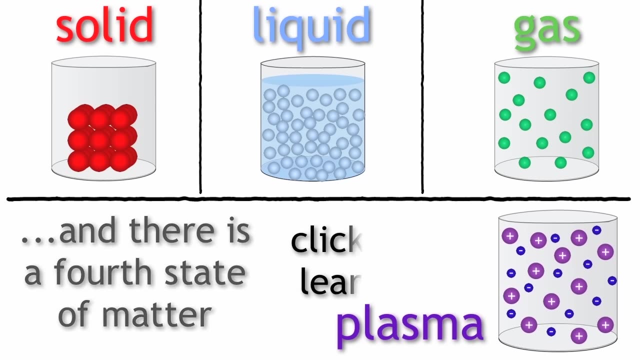 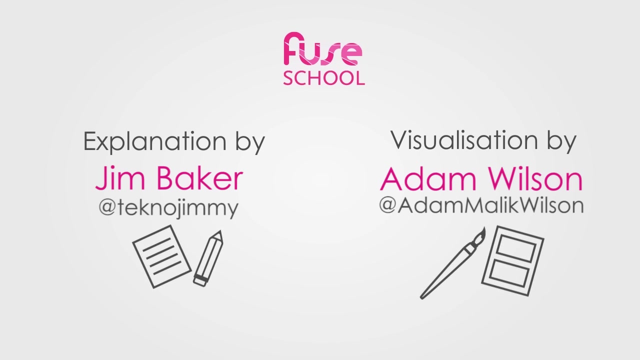 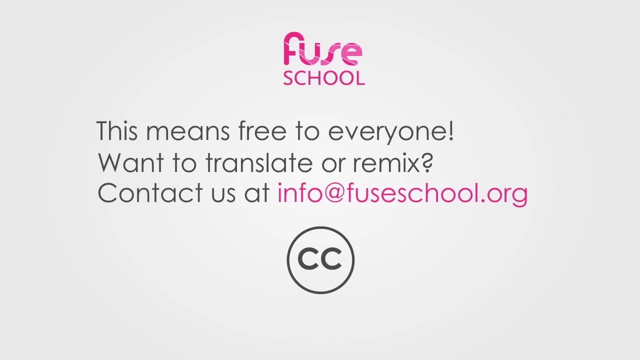 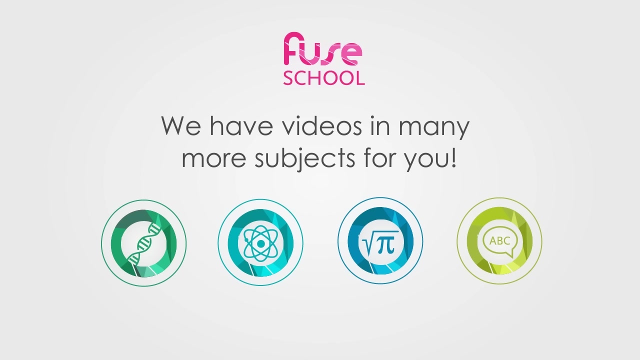 They do not have a fixed shape nor fixed volume. They fill the whole space they are in. That is why we call these gases gases. If you look at the original one, you will see that it is the same as a gas. Another example: a gas-like gas, because it is equal to a gas and it is less dense. 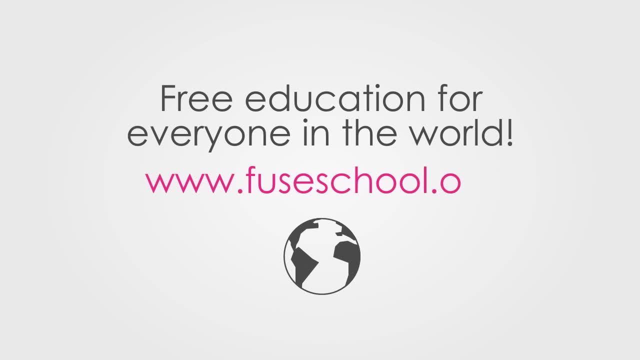 That is a gas-like gas. Here are two gas forms. This is the gas for liquid. We are going to apply this gas to the liquid. What I mean is that the gas forms are very small. You can see it now.